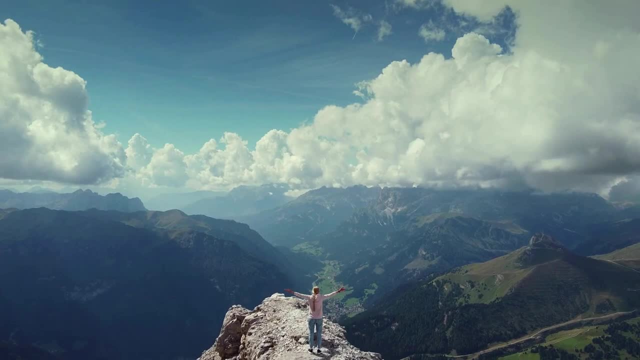 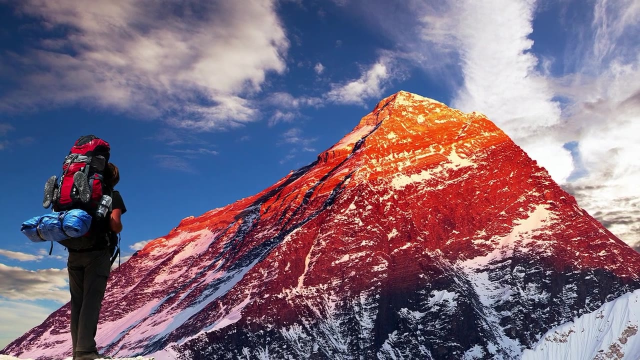 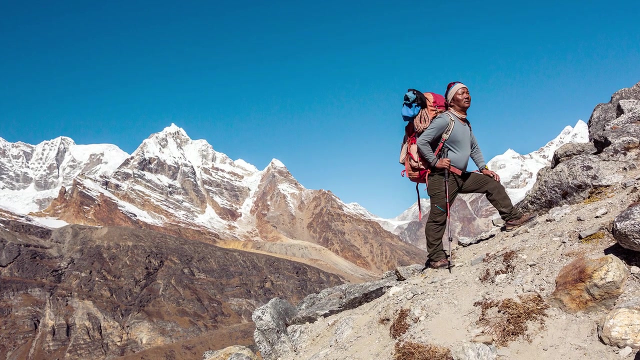 oxygen levels are low, it appears that humans' bodies can evolve over time to use more oxygen more efficiently. While most people would feel sick in the Tibetan mountains due to lack of oxygen, the bodies of the Tibetan people are oxygen converting machines. A euglena is a single-celled 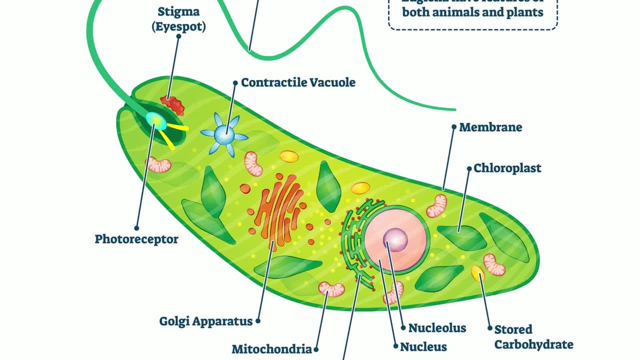 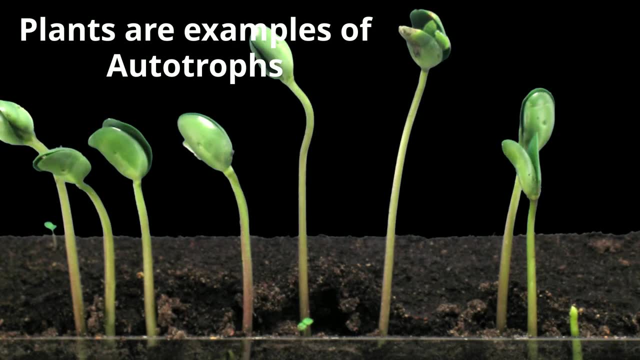 protist. These little protists adapted to become myxotrophs, meaning they can act as an autotroph and a heterotroph. Autotrophs are capable of producing their own food from inorganic substances. Euglenas are photoautotrophs. 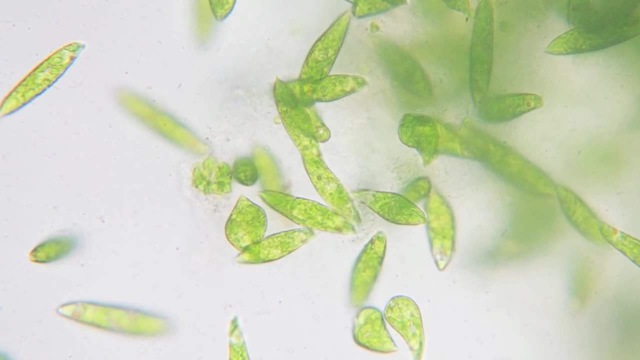 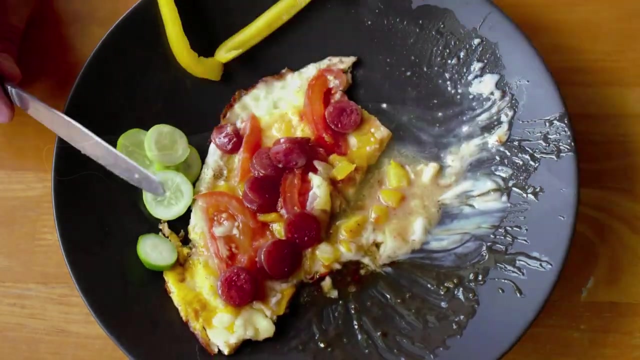 which means they have chloroplasts that allow them to carry out photosynthesis and make food from sunlight. Heterotrophs, on the other hand, must eat other organisms for food. Euglenas are also classified as heterotrophs because they feed on living organisms such as. 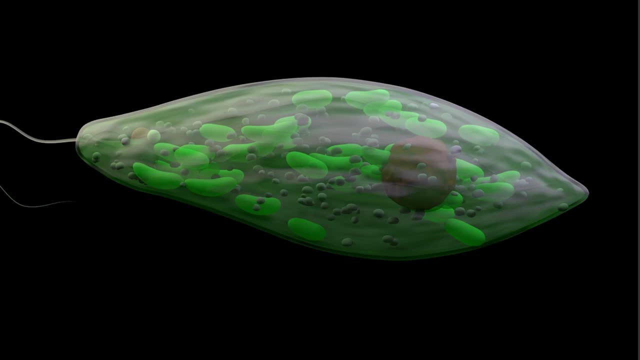 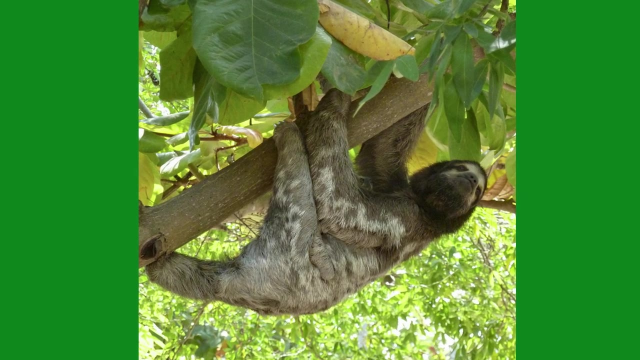 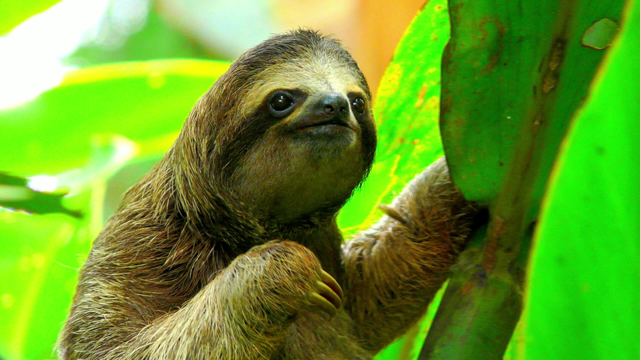 bacteria or algae. Sloths are famous for moving slow and hanging out in trees. They also have many adaptations that increase their fitness. For example, they have an extremely slow metabolism. Sloths' diet primarily consists of leaves. Leaves do not contain much energy, but a sloth's slow 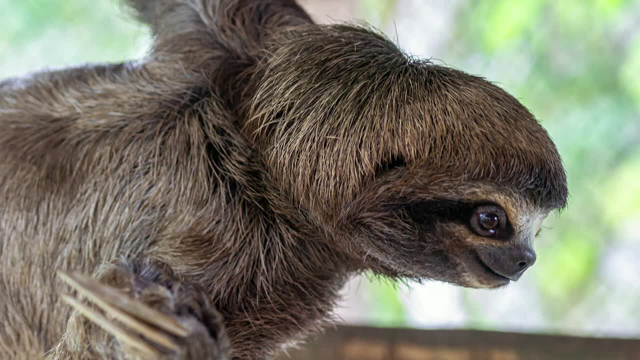 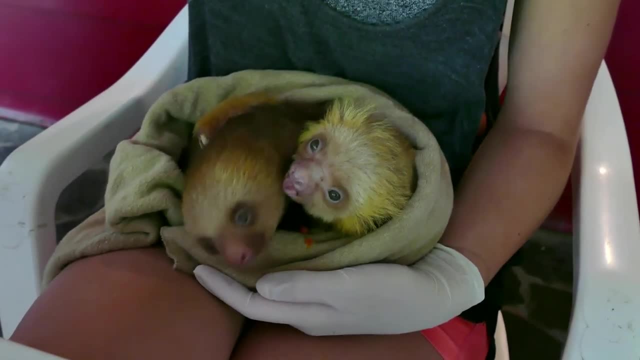 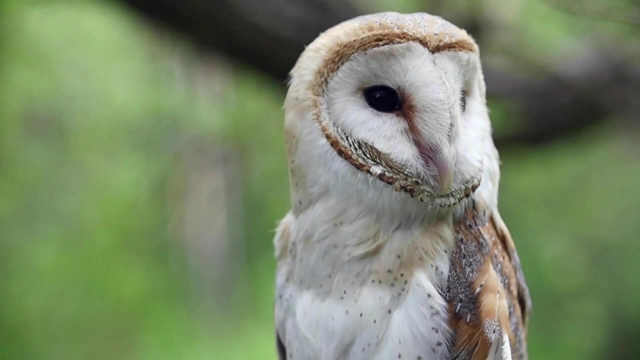 metabolism enables the sloth to store energy from its food for long periods of time. In addition, leaves are hard to digest, but sloths have a complex and rapid stomach that breaks down and ferments leaves efficiently. Owls are very successful birds of prey with many helpful adaptations. Here is a brief list. 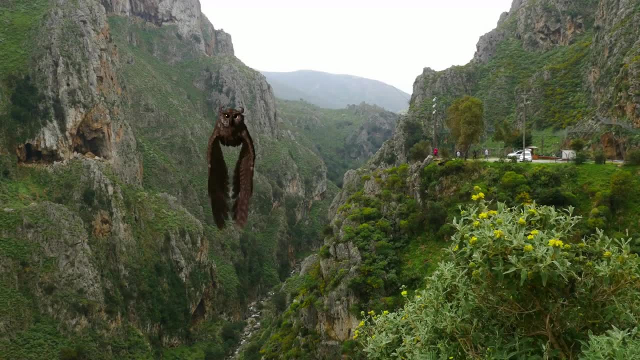 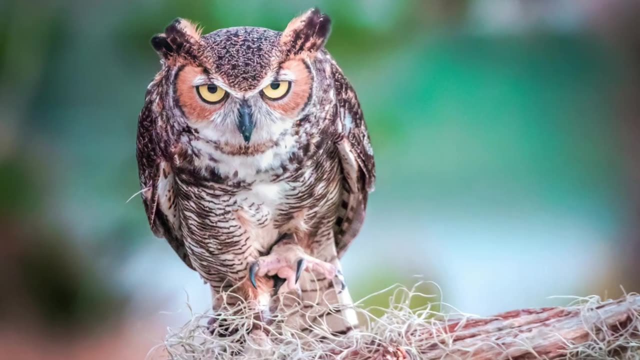 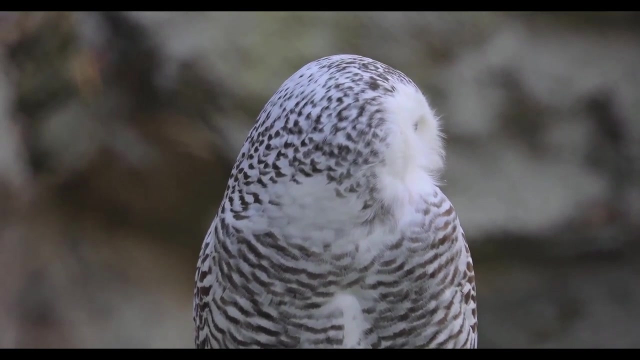 Their feathers are designed for silent flight. Their eyes are full of rods, which gives them extraordinarily good night vision. They have tufts that resemble twigs and branches And, finally, they have the ability to turn their heads about 270 degrees in each direction. You cant sneak up. 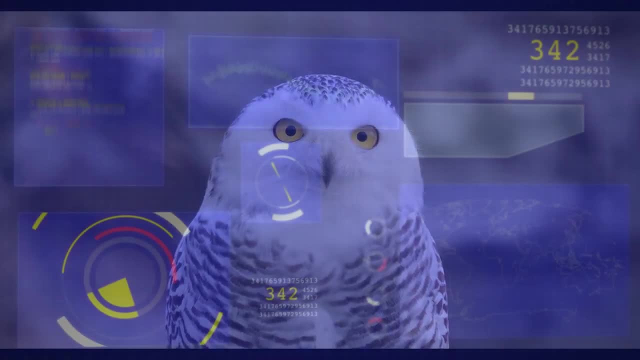 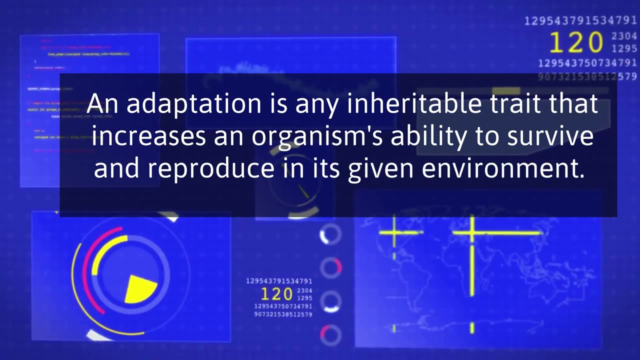 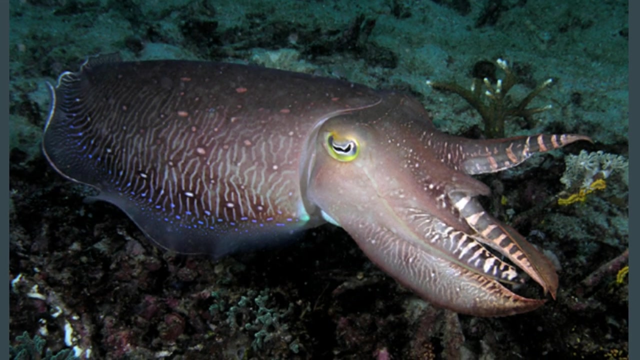 on an owl. Quick reminder: an adaptation is any inheritable trait that increases an organism's ability to survive and reproduce in its environment. Cuttlefish are masters of camouflage. They practice adaptive camouflage, which means they can change their color and texture based on their surroundings.